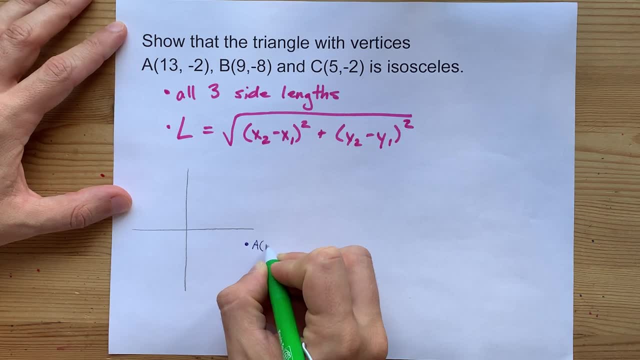 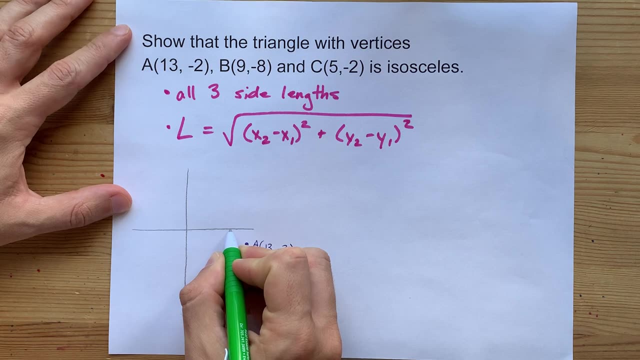 negative 2 on the y. so that is point A. Point B is at 9 comma, negative 8, so that's I don't know, 9 on the positive x and then negative 8 is way down here somewhere, 9 negative 8.. Lastly, C is at 5 comma, negative 2,. 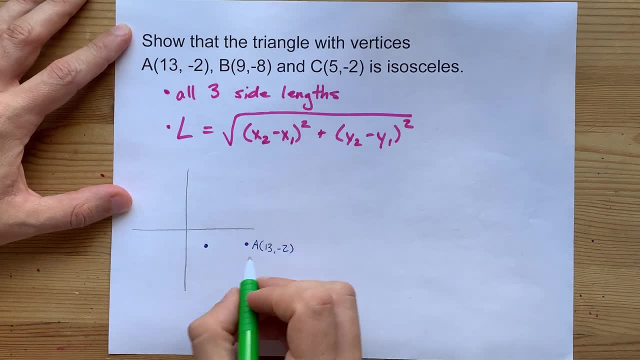 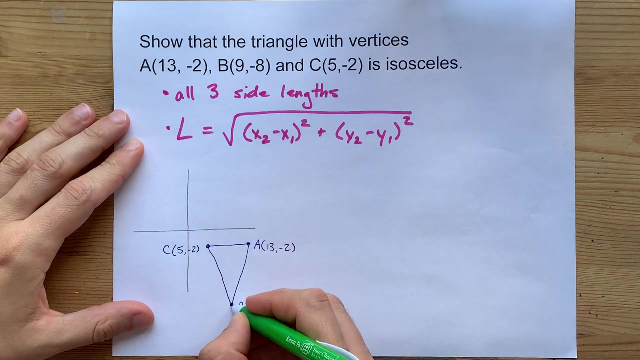 5 is going to be around here, comma negative 2.. Oh, those both have the same y value. well, that's going to be useful. C is at 5, comma negative 2.. Great, All right. so the triangle, the triangle itself, is here. What your job is: to prove that something is isosceles. 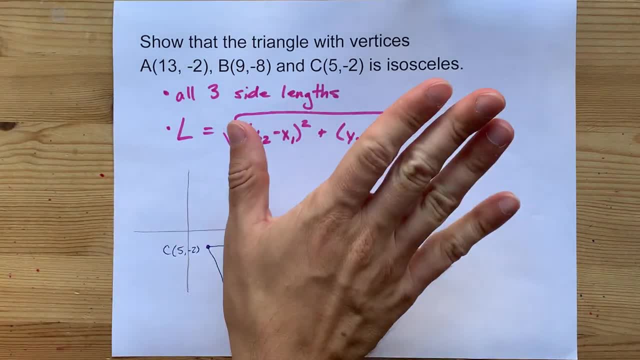 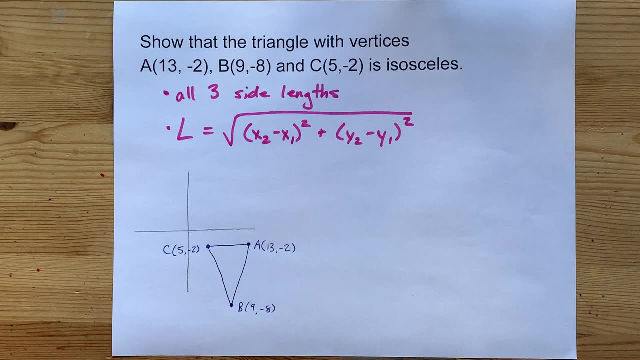 which means two sides of the same length or equilateral, all three the same length, or scalene, where none of them are equal. you're still going to have to do three length formulas. Let's together calculate the length between A and B. 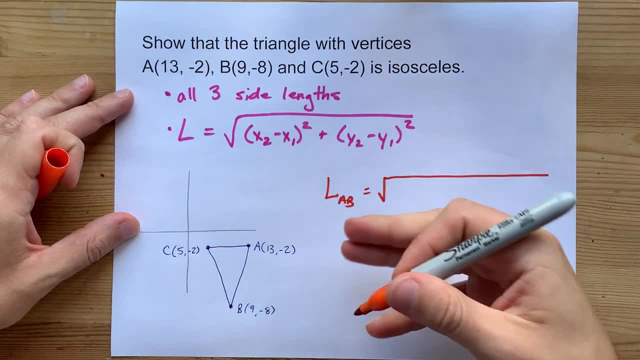 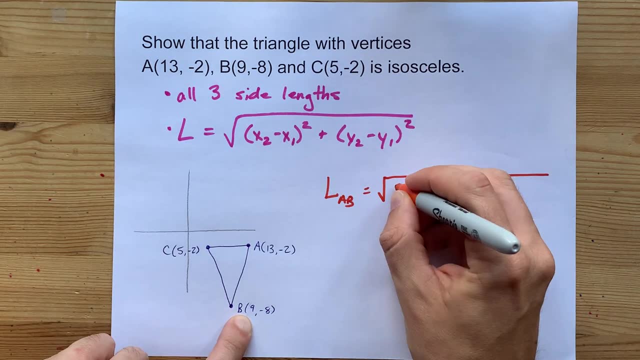 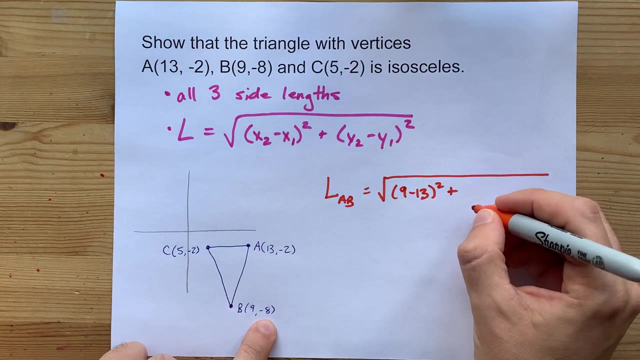 Now you might have to write out the whole formula for your teacher, but I'm just going to fill in the numbers. Now, if I'm going from A to B, then my x2 is 9,, my x1 is 13,, my y2 is negative 8,, my y1 is negative 2.. 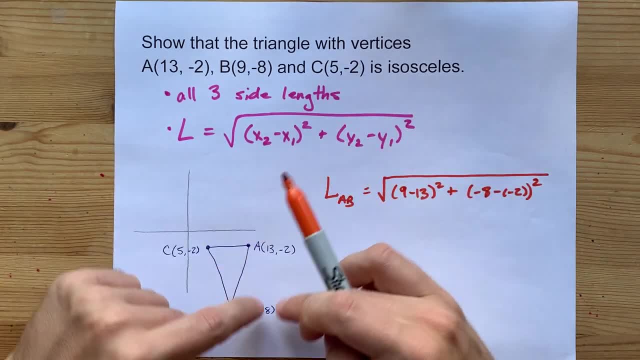 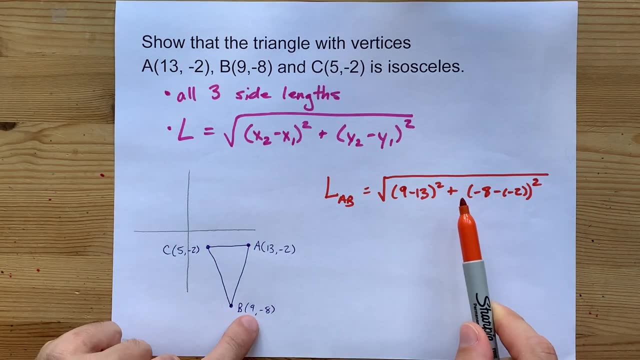 Now fun fact: in this formula, if you accidentally switch around which one is 2 or 1, it doesn't matter. just don't just make sure both your x's are first 9 and 13,, both your y's are next negative 8 and negative 2, that's what really matters. 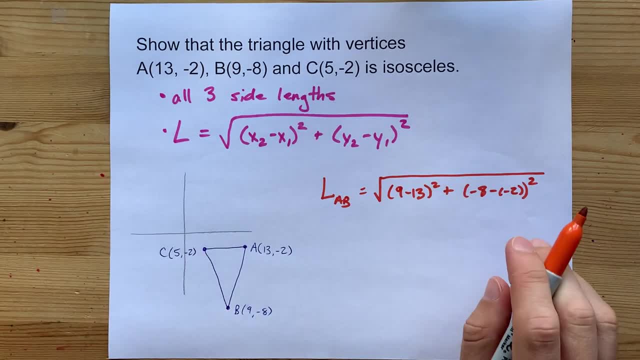 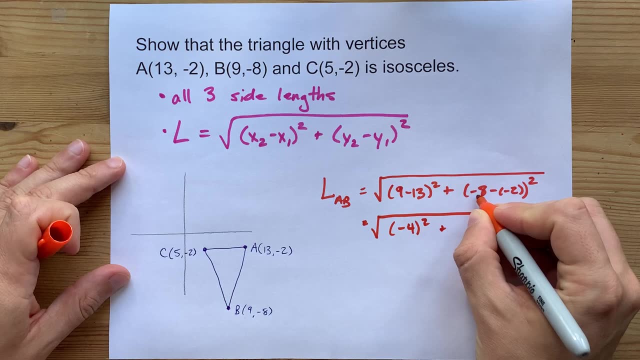 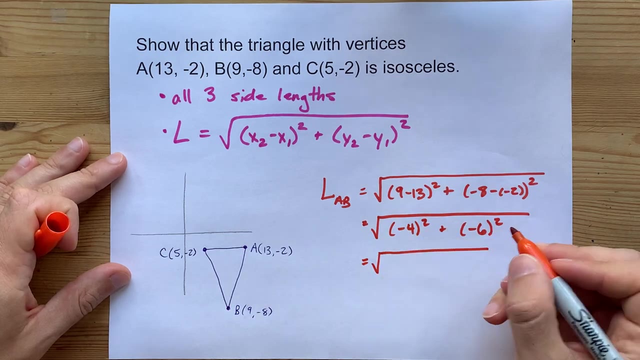 The squaring will get rid of any negatives that you accidentally cause to pop out. Anyways, 9 minus 13 is negative 4, negative 8 plus 2 is negative 6.. Now here comes the squaring: When you square a negative, it becomes positive. This is 16 and also. 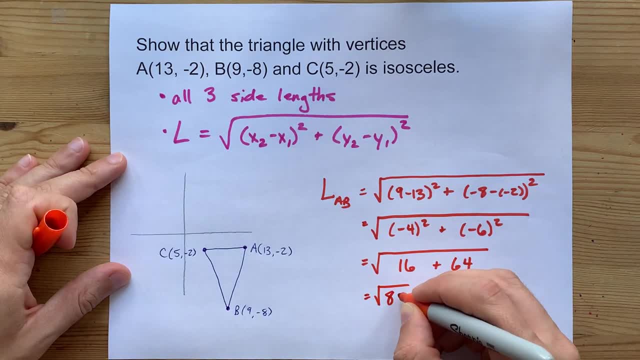 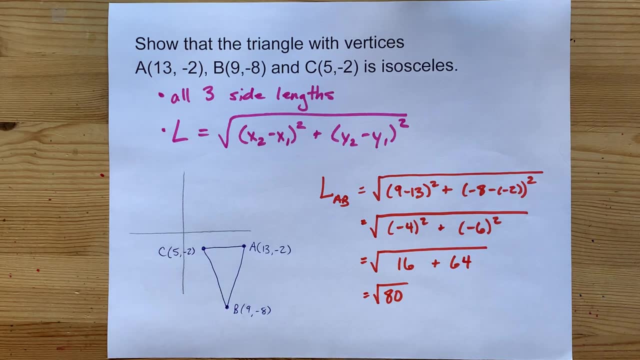 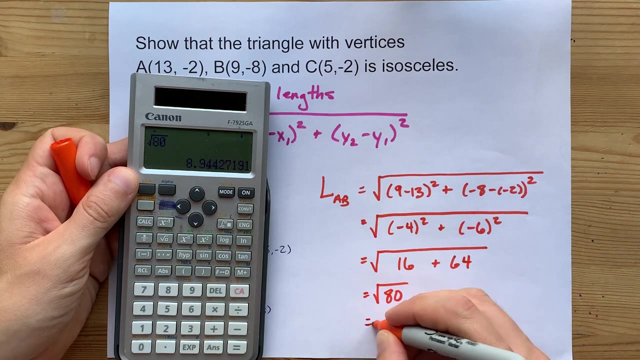 the square root of 80.. So 64.. That gives me the square root of 80.. Now that's what we call an exact solution, because you haven't done any rounding. But let's use a calculator somewhere and get the actual number for the square root of 80,: 8.944.. 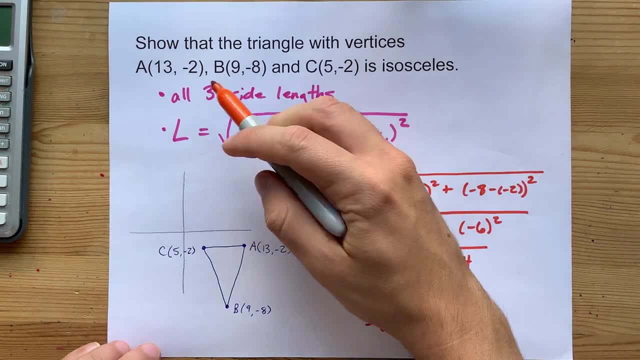 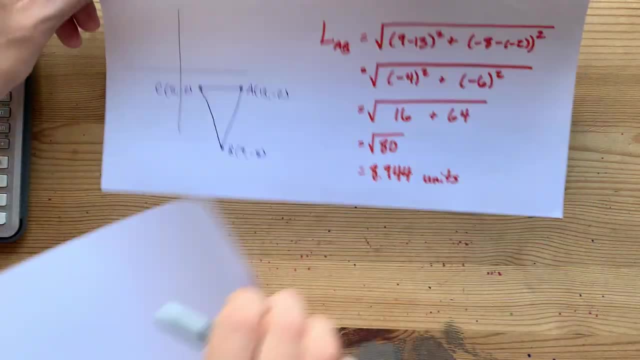 So the length from A to B is 8.944 units. We say units because we weren't given any actual units here. find from a to b. yes, i am personally going to do this for b to c and from a to c as well. that's a. 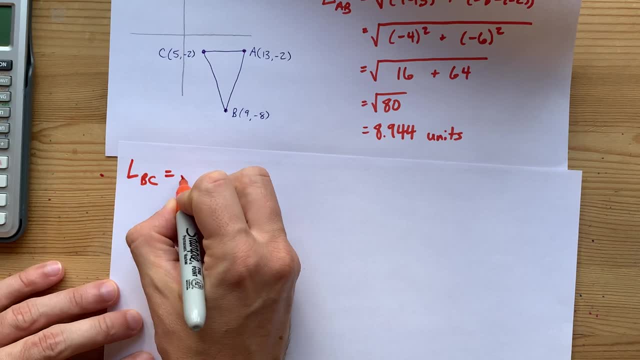 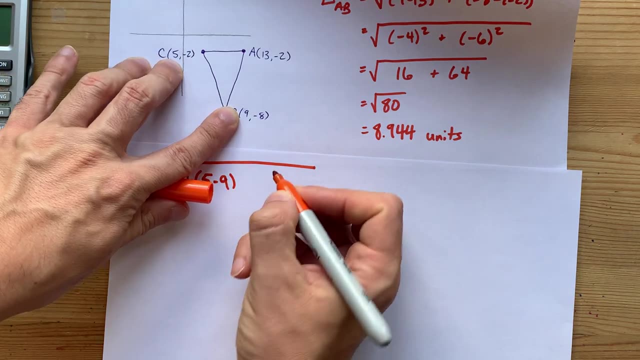 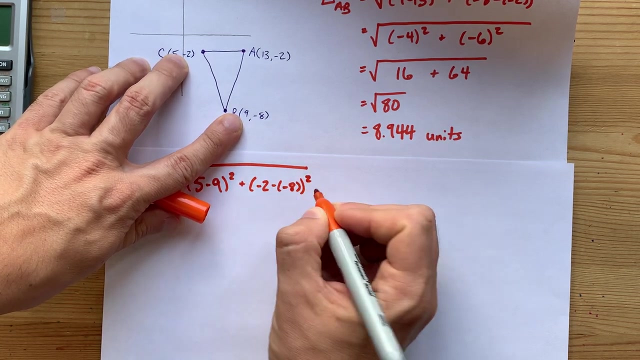 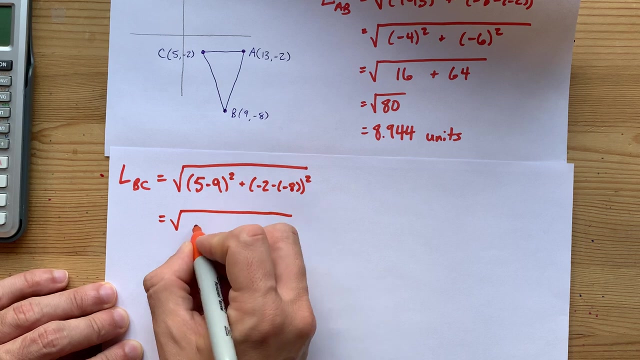 good height for you. the length from b to c: same deal b to c. we've got five minus nine for the two x's. we've got negative two minus negative eight for the two y's. see, i'm just taking them from the points themselves. let's calculate these square roots: five minus nine is negative four. 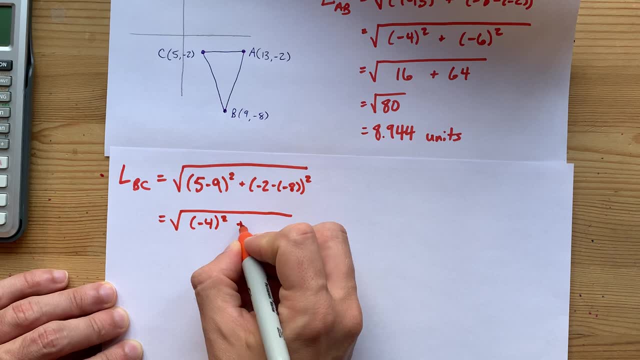 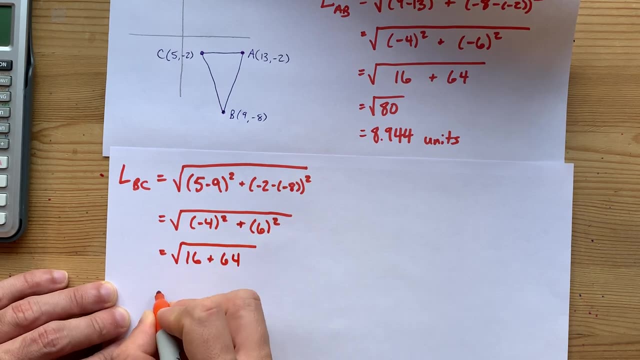 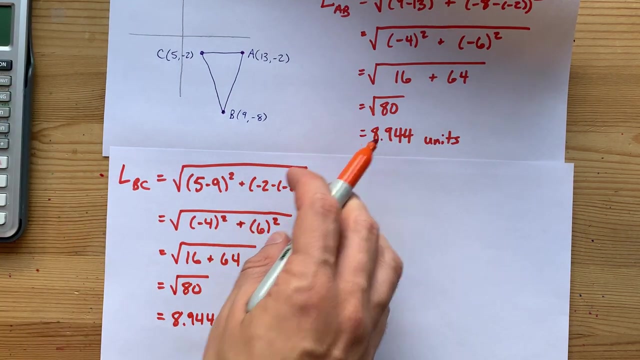 negative two plus eight is positive six. i like where this is going, because we get 16 and 64 again, so it's still root 80 again. that's the exact solution. the approximate solution is 8.944 units. cool, now i already noticed that AB and BC are the same length, so we're at least isosceles, but we have 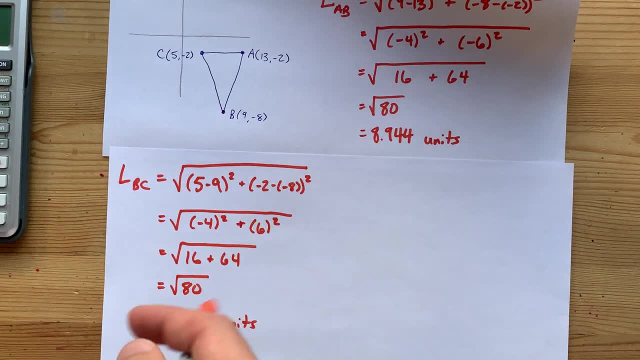 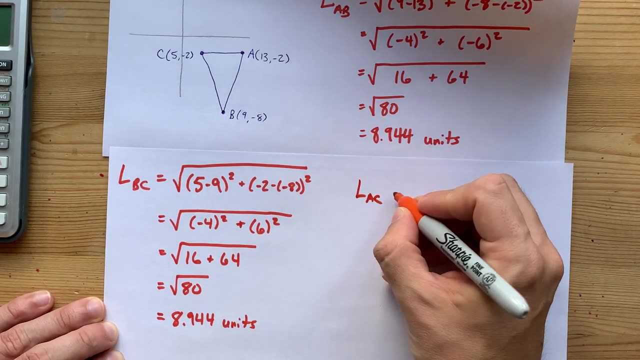 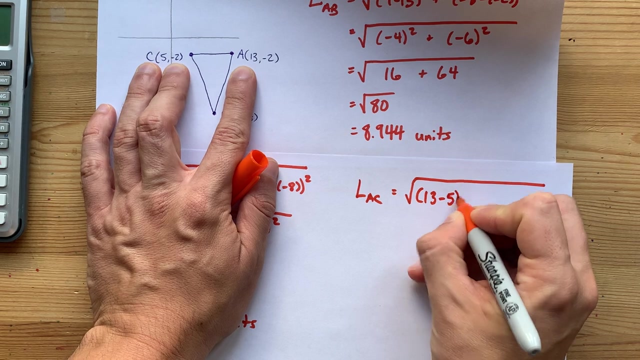 to check the third side. If the third side is the same length, it's actually scalene, not isosceles. So let's do it The length of AC, square root of A to C. We've got 13 minus 5 for our axes. 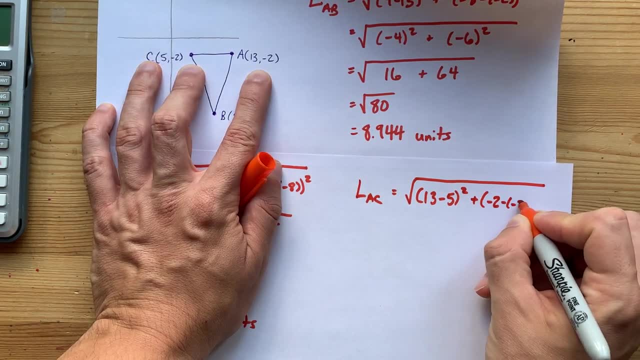 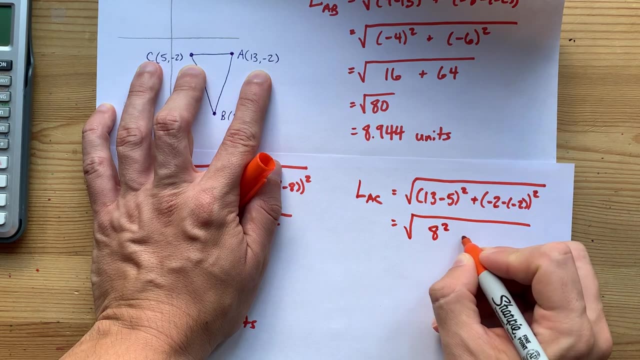 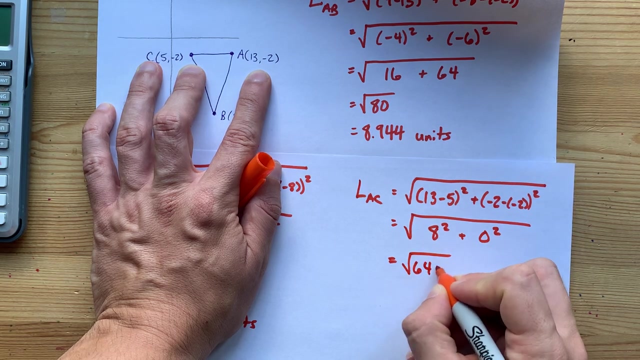 and we've got negative 2 minus negative 2. for our Ys These numbers are much different. 13 minus 5 is 8.. Negative 2 plus 2 is 0.. Oh, I see, It's the square root of 64, which itself is 8.. That is not. 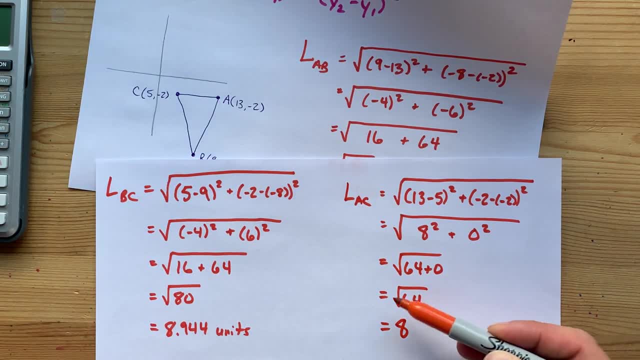 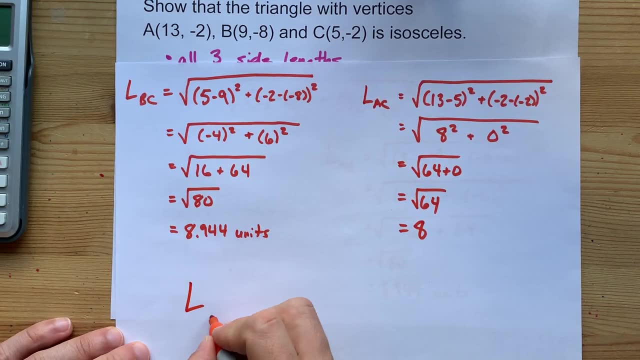 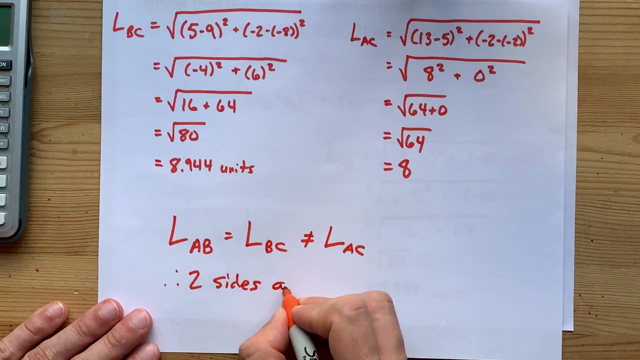 the same. Now here, 8 is the exact solution, because the square root of 64 is a nice round number. So what this means is that because the length of AB equals the length of BC, which is not the same length as AC, two sides are equal in length.